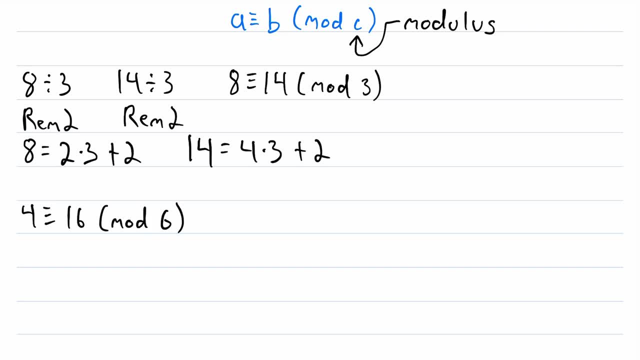 congruent to 16 mod 6.. We see this is true because 4 divided by 6 gives a remainder of 4.. 4 is equal to 0 times 6 plus 4.. And, of course, 16 divided by 6. 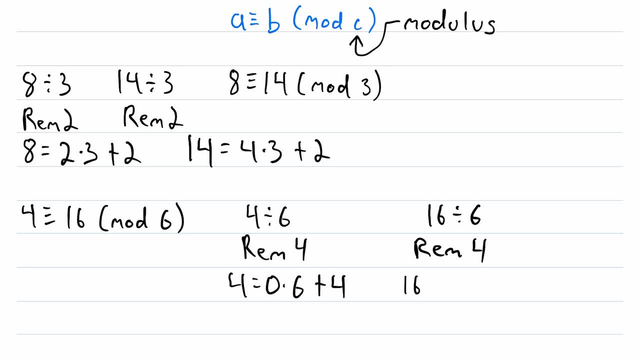 also gives a remainder of 4.. 16 is equal to 2 times 4 plus 4.. So again, this is true because 4 is congruent to 16 mod 3.. So times 6 plus 4.. So just as before, since 4 and 16 both have the same remainder when divided, 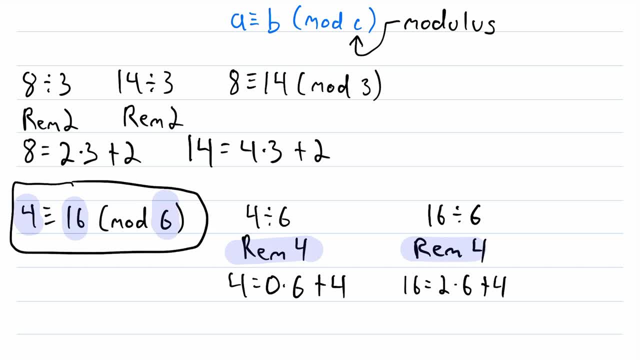 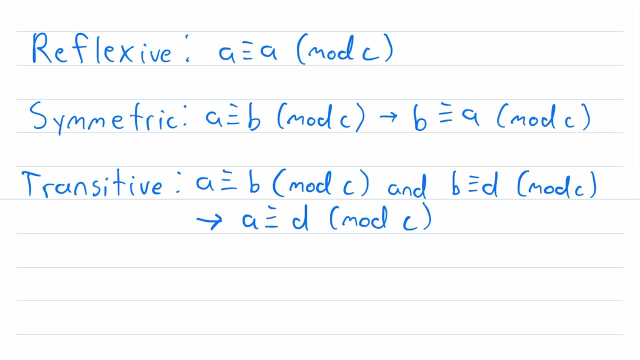 by 6, we say that these numbers are congruent mod 6.. Also, something important to note is that modular congruence is an equivalence relation. This means that modular congruence is reflexive, symmetric and transitive, So in many ways it works a lot like the equivalence. 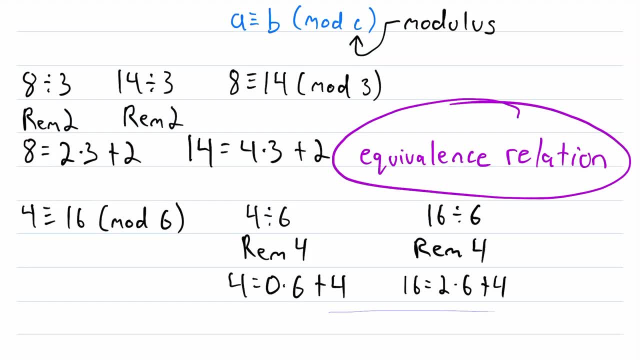 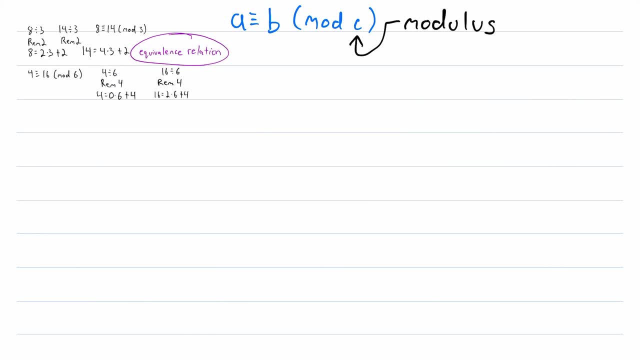 relation equal to that we're all very familiar with. But with all that said, let me shrink all this junk a little bit, move it out of the way, and then we can talk a bit more abstractly about modular congruence. And before we go on, I should add that when we're talking about modular congruence, 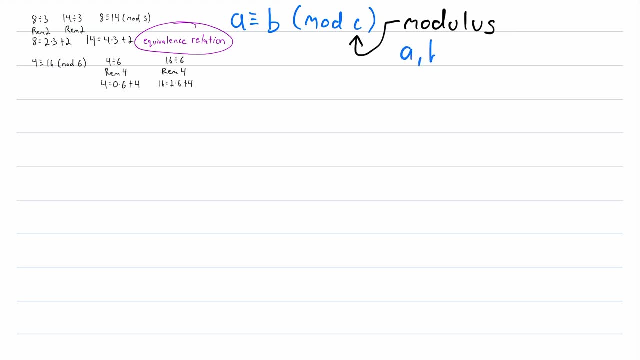 a and b are usually going to be integers, so a and b are elements of the integers and c, the modulus, is a natural number greater than 1.. So c is an element of the natural numbers and c is greater than 1.. 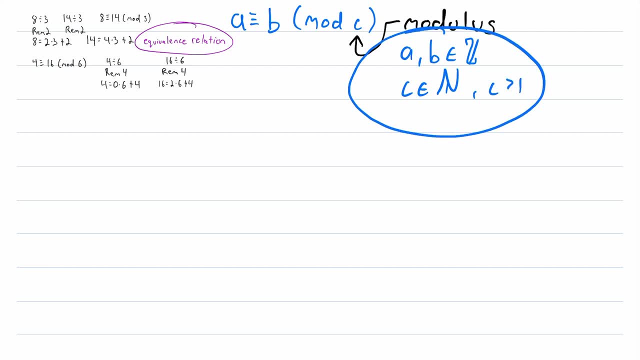 So most often these are the types of numbers we're talking about with modular congruence. We already said that a is congruent to b mod c if, and only if, a and b have the same remainders when divided by c. But there's also another equivalent definition of modular congruence: 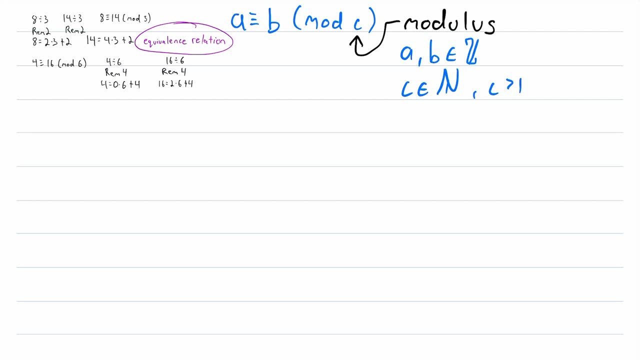 that is often used and often useful. This other definition says that a is congruent to b mod c if, and only if, c divides a minus b. So mod c is congruent to b mod c if, and only if, c divides a minus b. So if, and only if, c divides a minus b. 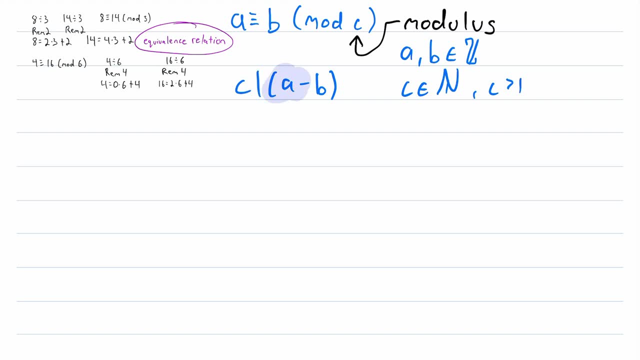 This notation c divides a minus b just means that a minus b is an integer multiple of c. The two definitions we have stated are equivalent definitions, but I think this one is a bit less ambiguous because the other definition uses the word remainder, and people don't always mean the 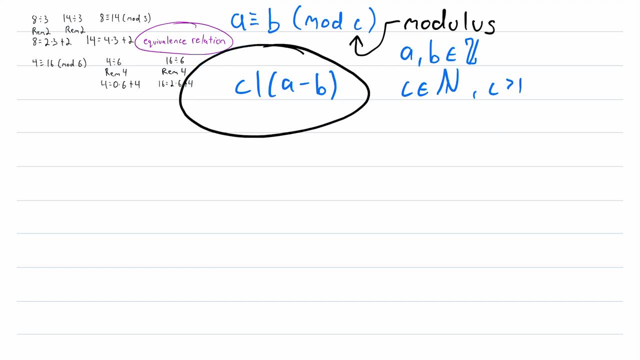 exact same thing by the word remainder. So let's see this definition in action. We already said that 8 is congruent to 14 mod 3.. Then 3,, which is our c value, should divide 8 minus 14,, which are our a and b values respectively. So is that true? 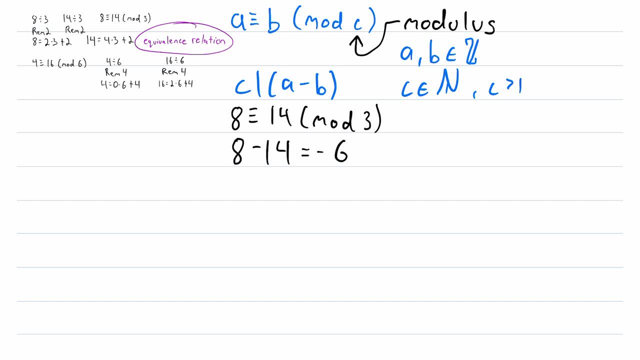 Well, 8 minus 14 is equal to negative 6.. And indeed 3 does divide negative 6, because negative 6 is an integer multiple of 3.. We can see that because negative 6 is equal to 3 times negative 2.. Now let's see an example of using this definition to establish modular congruence. Consider 23 minus 9.. 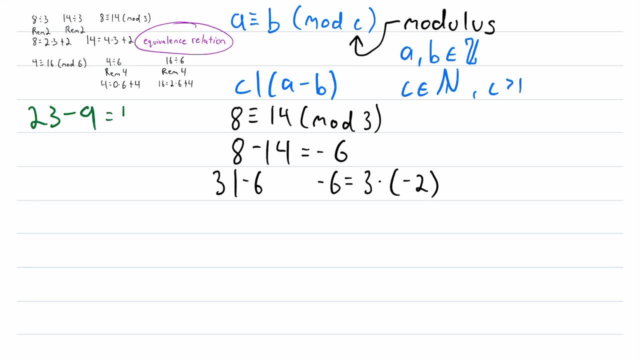 Now let's see an example of using this definition to establish modular congruence. Consider 23 minus 9.. 23 minus 9 is equal to 14, and we know that 7 divides 14 because 14 is equal to 7 times 2.. 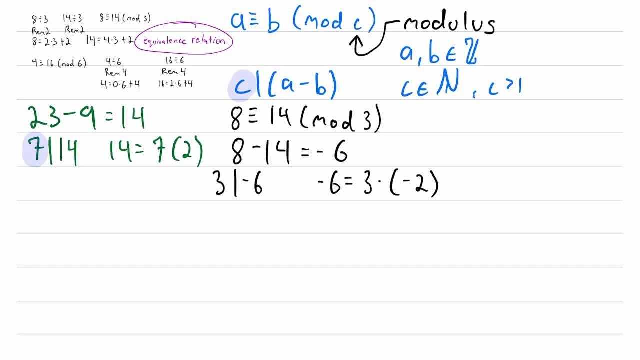 So, since 7, our c value in this case divides 23 minus 9, our a and b values respectively, that means that 23 is congruent to 9 mod 7.. Additionally, since 2 divides 14,, we could also say that 23 is congruent to 9 mod 7.. 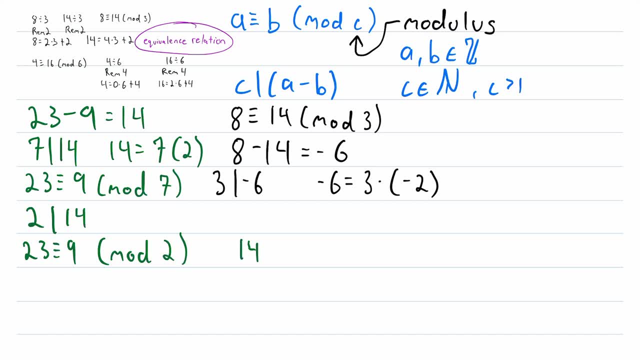 Additionally, since 2 divides 14, we could also say that 23 is congruent to 9 mod 7.. Additionally, since 2 divides 14, we could also say that 23 is congruent to 9 mod 7.. 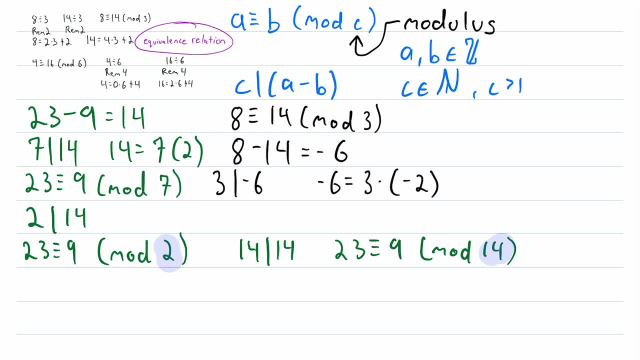 Again, this is because 14,, 2, and 7 all divide 23 minus 9.. To refer back to the first definition we stated: 23 divided by 14 has a remainder of 9, and 9 divided by 14 also has a remainder of 9.. To refer back to the first definition, we stated: 23 divided by 14 has a remainder of 9, and 9 divided by 14 also has a remainder of 9.. To refer back to the first definition, we stated: 23 divided by 14 has a remainder of 9, and 9 divided by 14 also has a remainder of 9.. 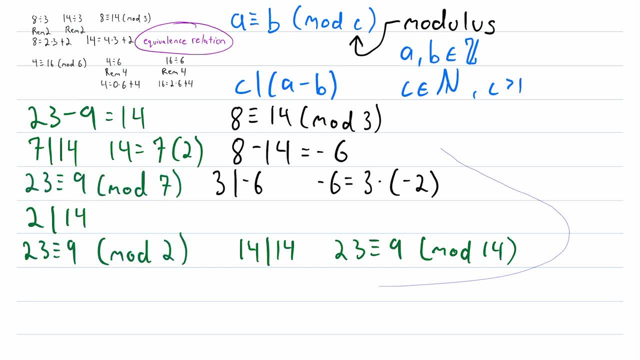 To refer back to the first definition, we stated: 23 divided by 14 has a remainder of 9, and 9 divided by 14 also has a remainder of 9.. with these other examples? So those are just a few more examples of modular congruence. 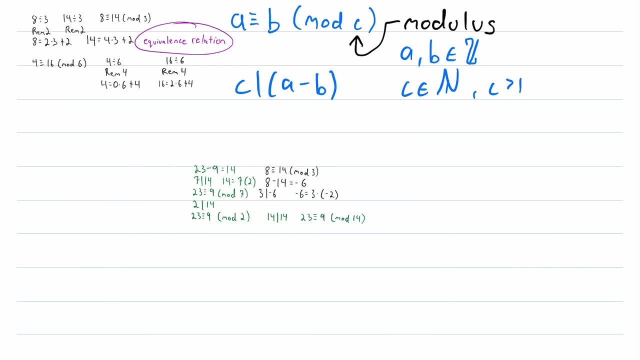 using this other definition. Let me shrink all this stuff down a little bit And I'll I'll hide this up here, sneak it up here in the corner. I think we should briefly touch on modular congruence with negative numbers before we go. So here is an example of that. 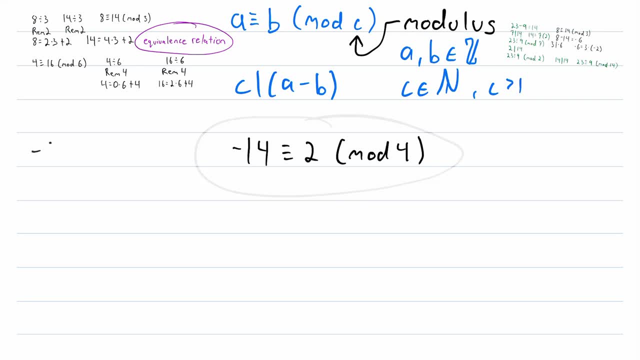 Negative 14 is congruent to two mod four, because negative 14 minus two is equal to negative 16.. And four does divide negative 16, because negative 16 is equal to four multiplied by negative four. But what if we were using the other definition that involves remainders. 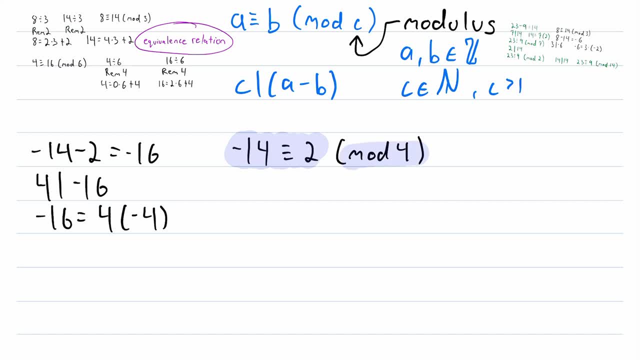 How would we be able to conclude that 14 is congruent to two mod four using that definition? Well, what is the remainder of negative 14? When divided by four, the remainder in this case is positive two, because negative 14 is equal to four. 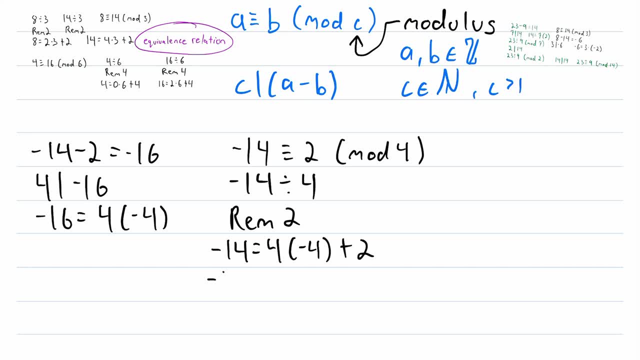 mod four. Well, what is the remainder of negative 14 when divided by four? The remainder in this case, is positive two, because negative 14 is equal to four mod four multiplied by negative 4 plus 2.. And you might be thinking- well, wait a minute. negative 14 is also equal to 4 times negative 3. 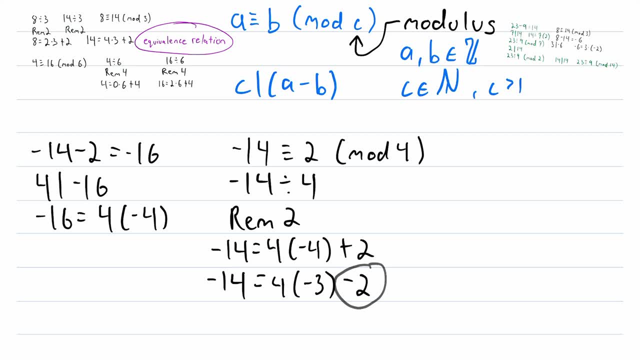 minus 2.. So why isn't negative 2 the remainder? Well, in this context, if we have a number a divided by c and we want to know the remainder, r, we want r, the remainder, to be greater than or equal to 0 and less than c. So we consider the remainder to be a. 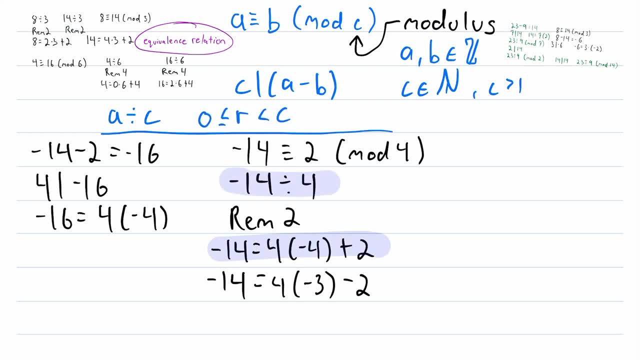 positive number, And that's why positive 2 is the remainder in this case and not negative 2.. And then, of course, if we take 2 divided by 4, just to finish this example, we have a remainder of 2, because 2 is equal to 4 multiplied by 0 plus 2.. So that's just a 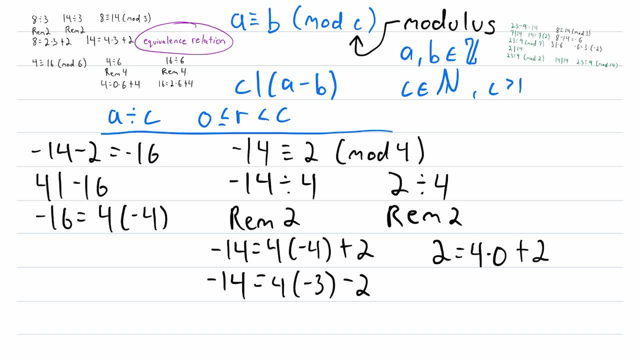 little bit about modular congruence. As a quick recap, we say that a is congruent to b mod c if, and only if, a and b both have the same remainder when divided by c. Equivalently, a is congruent to b mod c if, and only if, c divides a minus b. There is a lot more we could get into regarding modular. 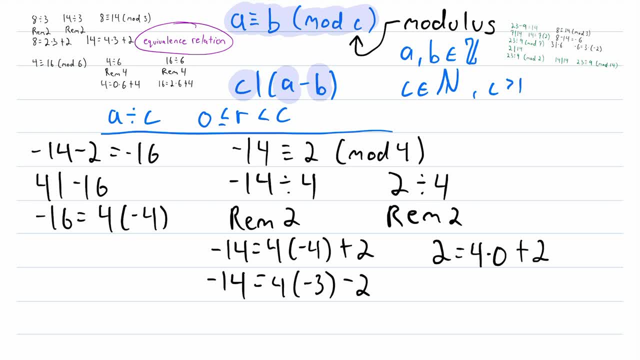 congruence, like modular arithmetic and all sorts of useful properties regarding modular congruence, But for now we'll call it a day, so I hope this video helped you understand what modular congruence is. Let me know in the comments if you have any questions, need anything.